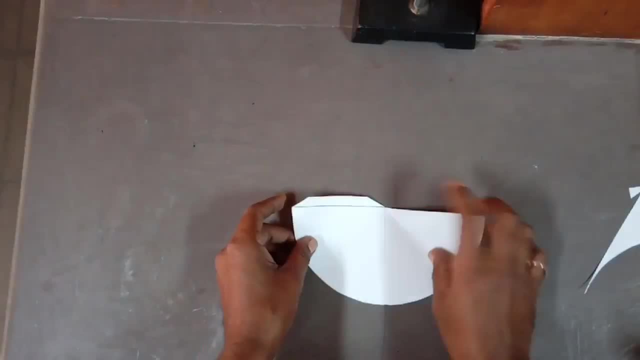 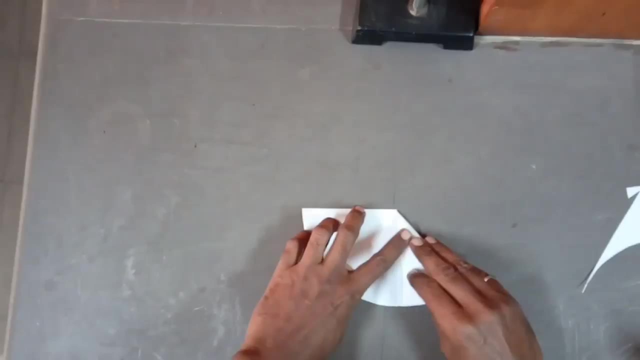 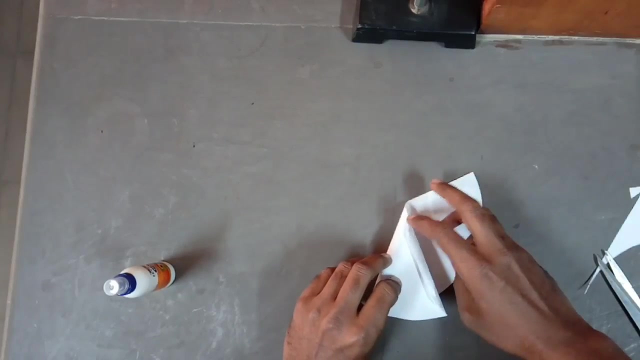 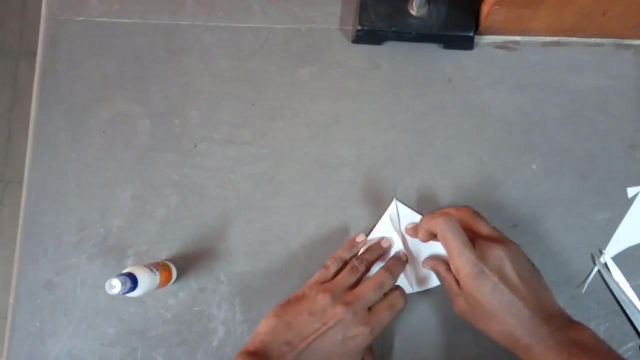 will act as the flap to join the cone. now fold the margin. this will act as flap. now bring both the radius at the semicircle of the semicircle on the mid line and apply glue over the flap and stick it over the other part. now hold it. 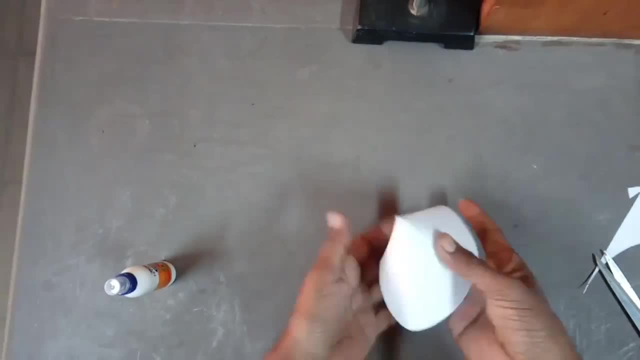 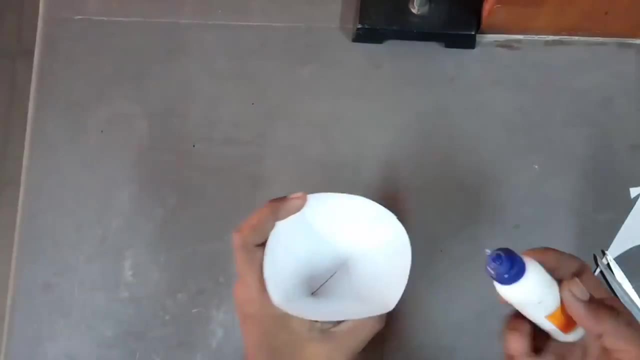 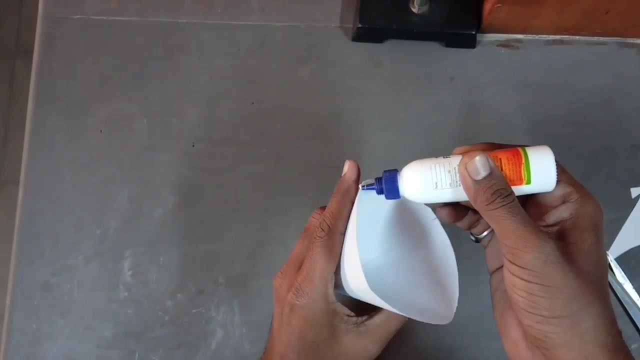 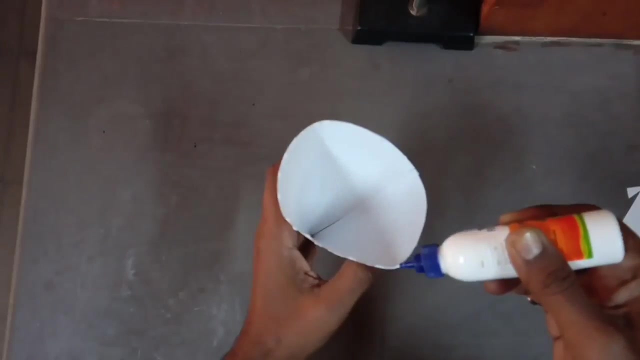 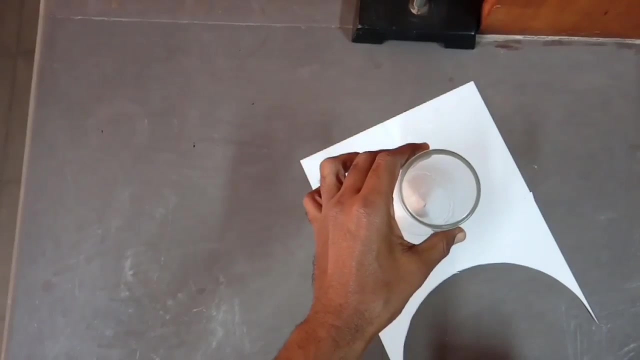 for few seconds to fix them. do not press the corners as the or the slanted edges now apply fevicol over its circumference and put it over remaining part of the sheet and put a inverted glass over it due to the weight of the glass, our cone. 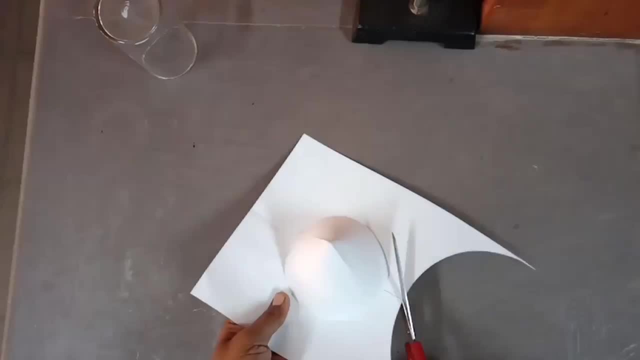 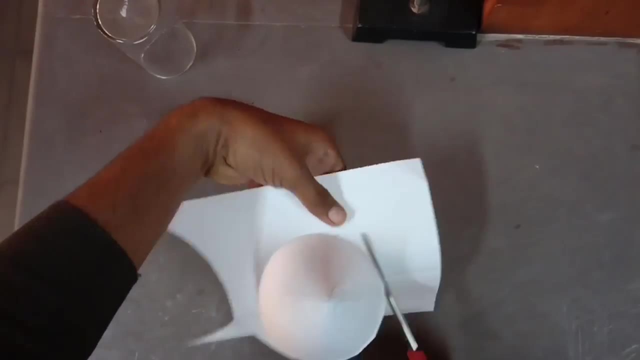 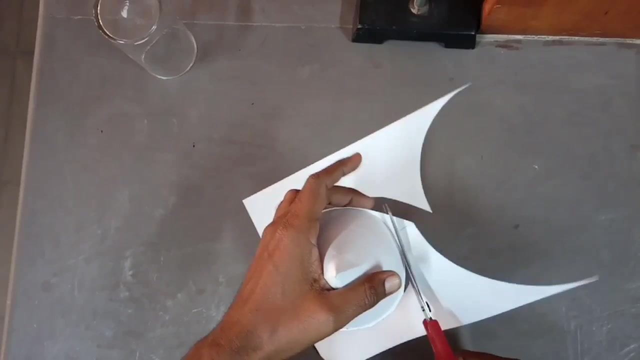 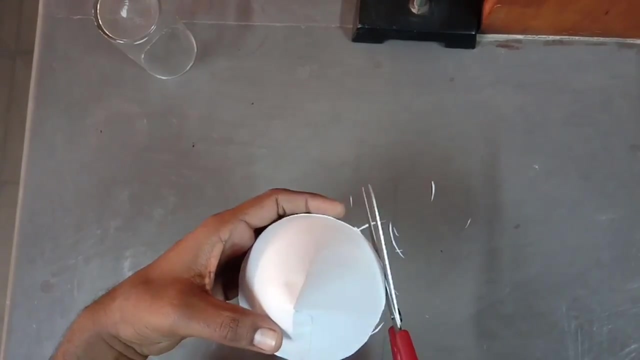 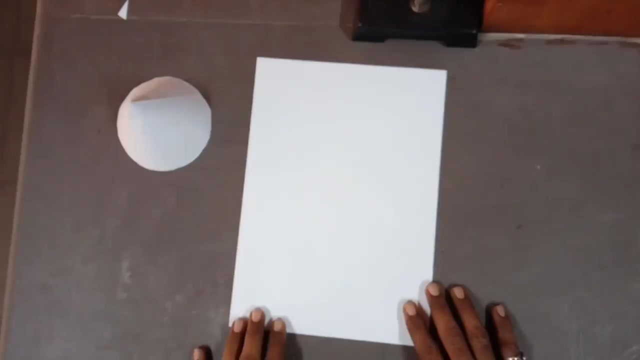 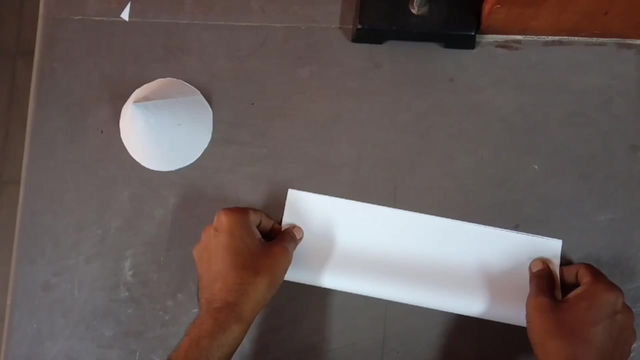 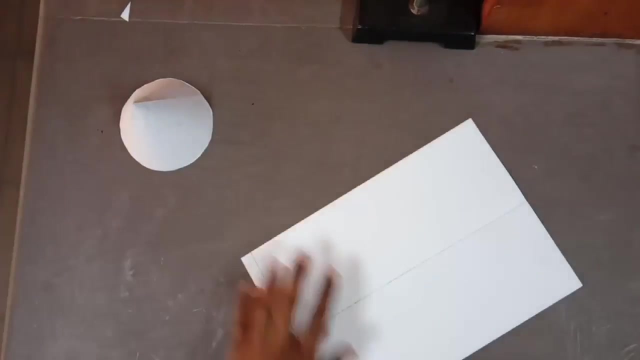 will automatically take a perfect round shape. wait for few minutes and cut the extra sheet. try to make it perfect round. in this way, a very beautiful right circular cone is ready with its pace. similarly like this, we can make cones of different height and radius. you just have to increase or decrease the radius of the circle, like this time. 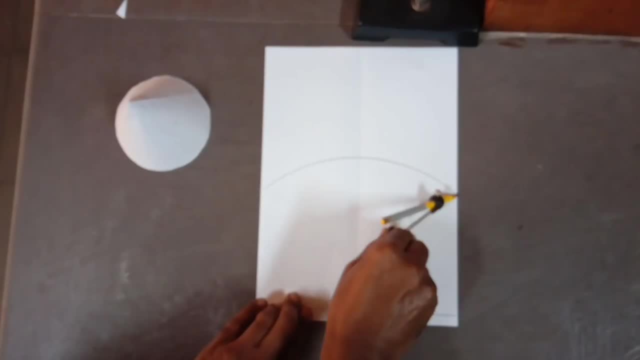 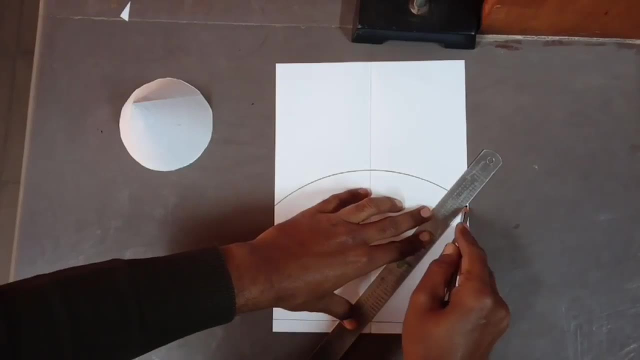 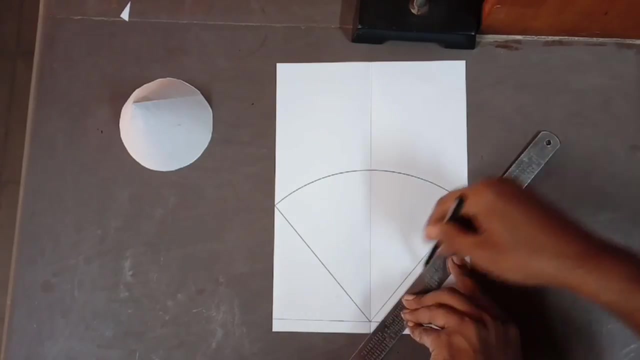 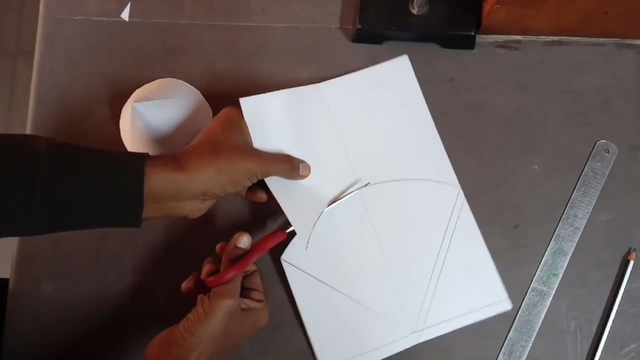 when we increased the radius of the circle. we are getting a small sector of a circle, this time our previous border, since we just floors an existing one. so we thought we may go ahead and fill up the TERRAD round shape now, if you are useless, so make a fresh margin along one of its edge and cut out this sector of.